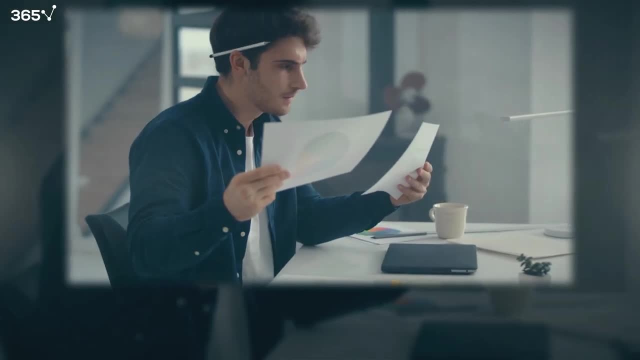 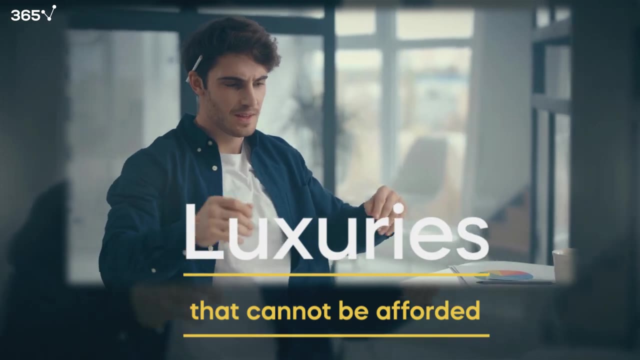 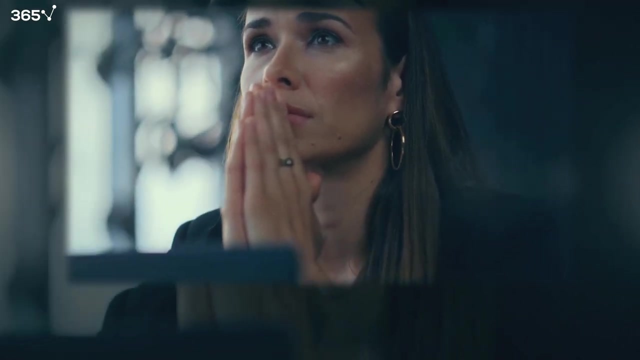 and a bottom line in red. startup founders and small business owners in general feel that investment in data strategy, data collection and data analysis is a luxury that they simply cannot afford, because they need to dedicate their energy on actions that will produce results now rather than in a year. This mindset is reminiscent of Gil Amelio, who was Apple's CEO before. 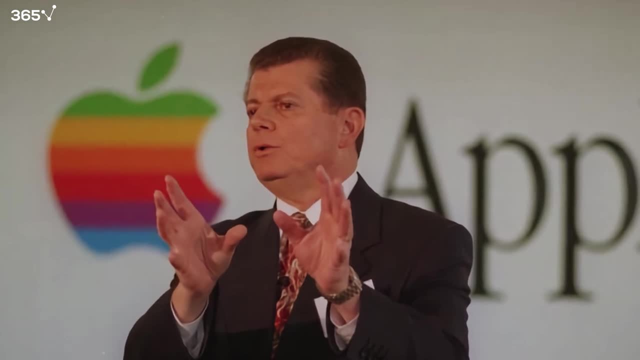 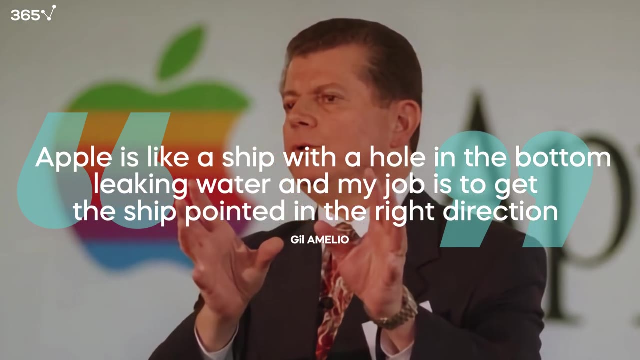 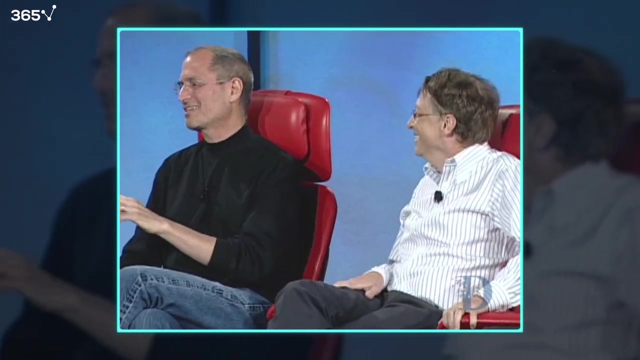 Steve Jobs took over. In a question on how the tech company was doing, he famously said: Apple is like a ship with a hole in the bottom leaking water, And my job is to get the ship pointed in the right direction. Gil was a nice guy but he had a saying. He said: Apple is like 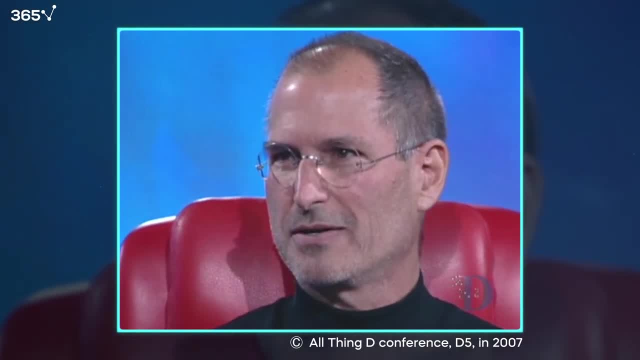 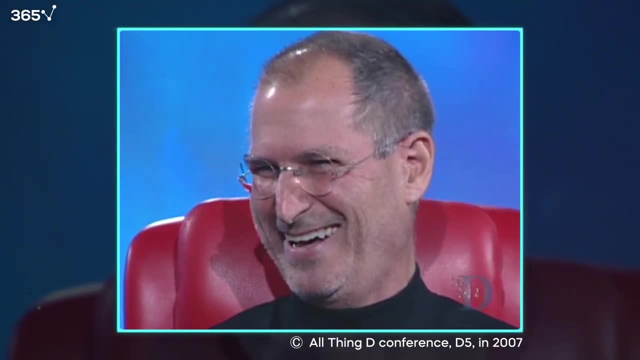 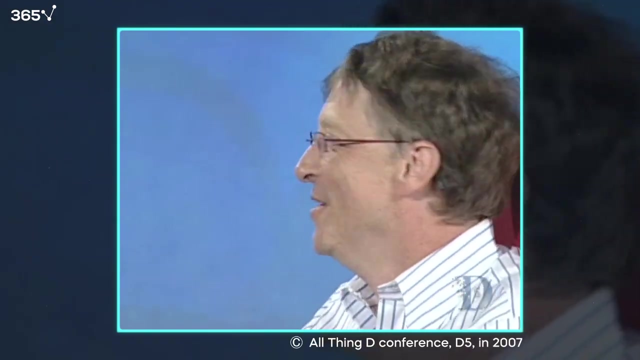 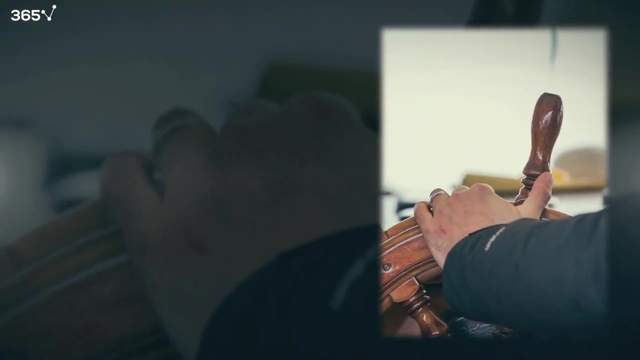 a ship with a hole in the bottom leaking water, And my job is to get the ship pointed in the right direction. If you're the captain of a ship that's leaking water, would you try to point it in the right direction Or would you try to do something about the hole in its structure instead? 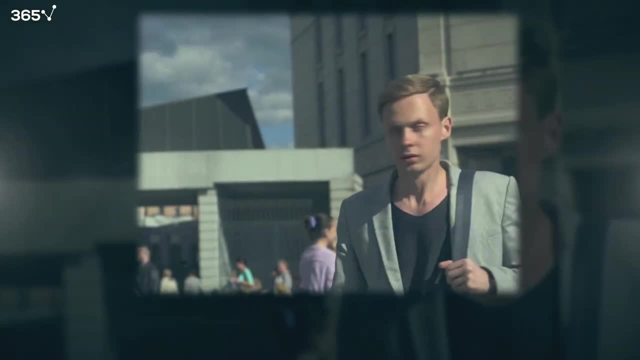 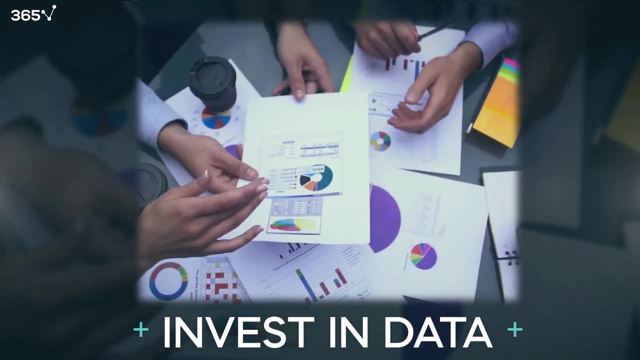 Similarly, if you run a business without knowing where exactly you're headed, would you continue to work harder but be essentially blind to growth? Or should you invest in a new business, Or should you invest in data that will point you in the right direction? 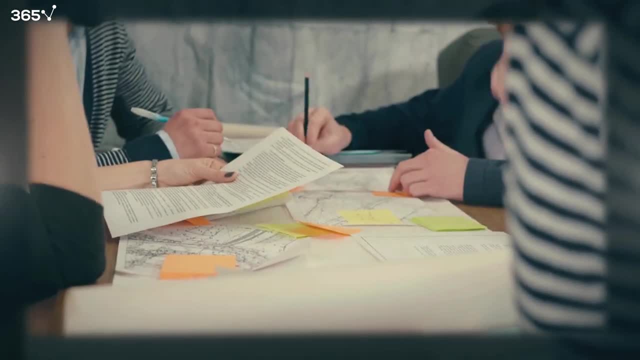 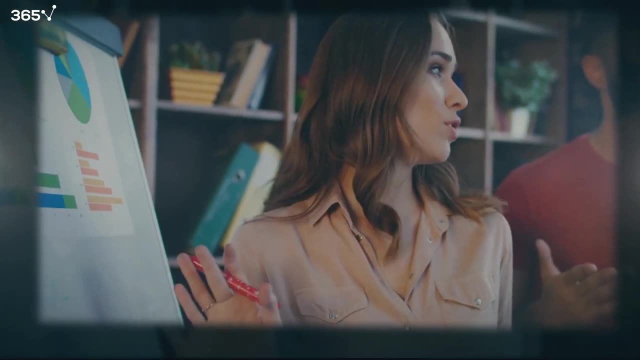 Yes, small businesses have very scarce resources, and it is precisely why they cannot afford to waste any of them. The only way to ensure that they make the most out of what they have is to adopt data-driven decision-making. At this point, you might be asking: can all small businesses? 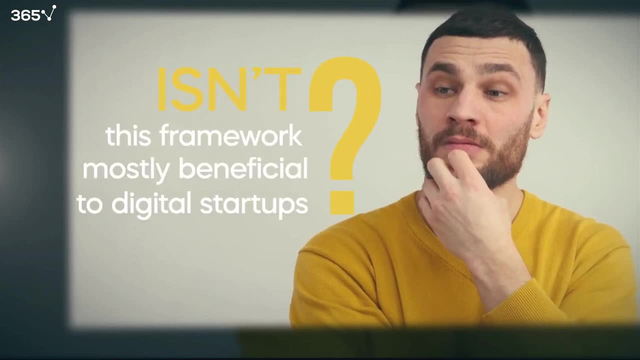 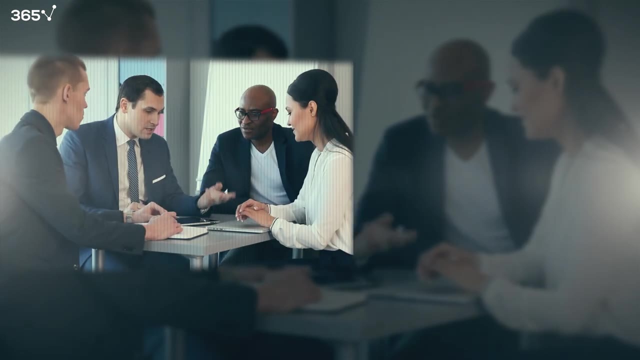 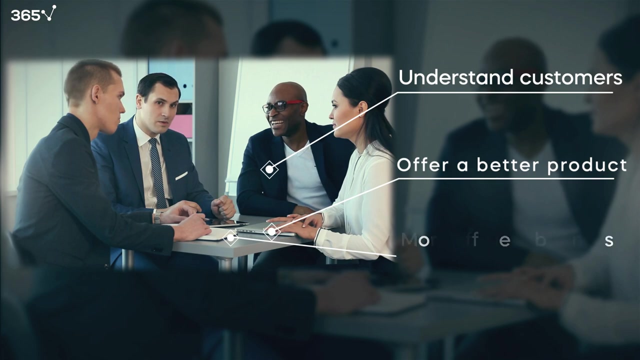 benefit from data. Isn't this framework mostly beneficial for digital startups rather than traditional firms? That's a common misconception. In reality, if your company needs to understand its customers and find ways to offer a better product, or if you are interested in running a business that is more operationally efficient, 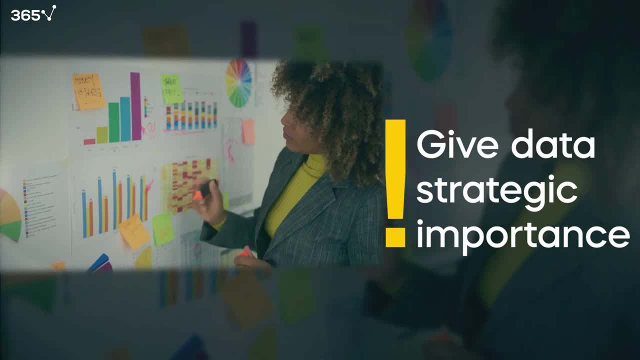 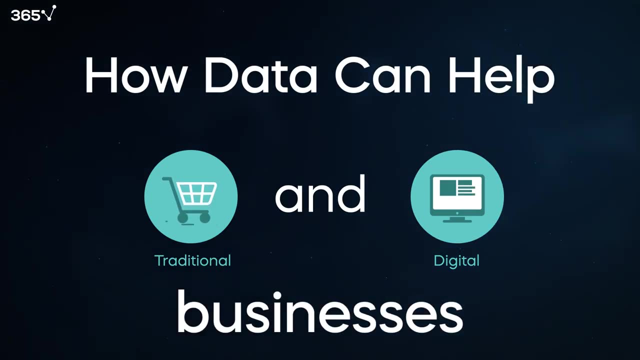 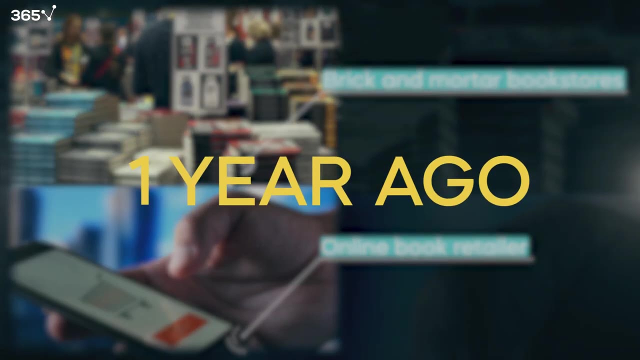 then you certainly need to give data strategic importance. Let's see how data can help a traditional and a digital business respectively, through a real-world scenario. Consider a chain of three brick-and-mortar bookstores and an exclusively online book retailer, all of which started operating a year ago. 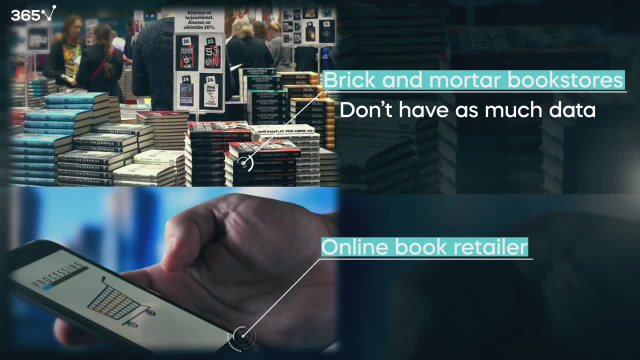 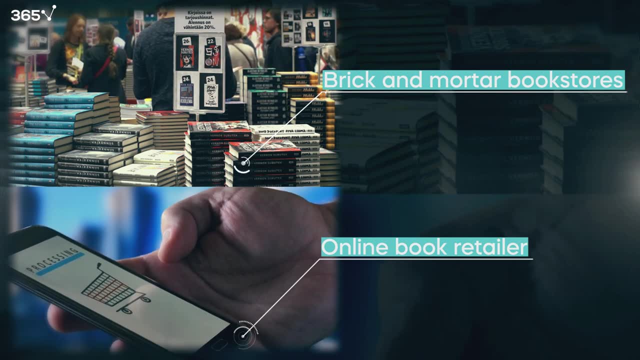 Presumably the brick-and-mortar stores do not have as much data as the digital business, which puts them at a slight disadvantage. Nevertheless, management has multiple options to utilize data and begin collecting insights. What they can do is place sensors that detect. 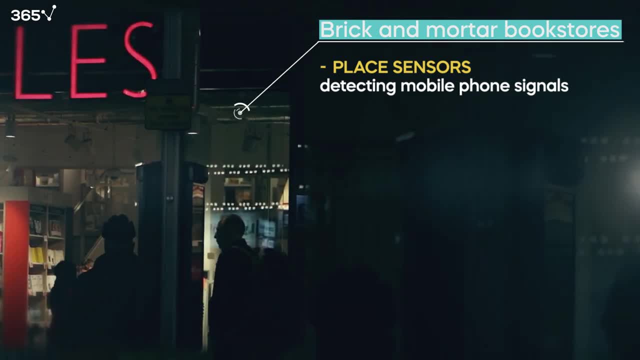 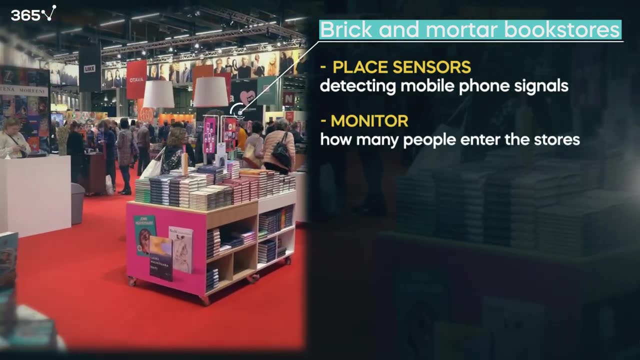 mobile phone signals on shop windows to collect information on footfall, to ensure stores are in areas with sufficient customer traffic. Monitor how many people enter the stores in order to experiment with promotional messages And different arrangements of shop windows to try and attract more engagement. 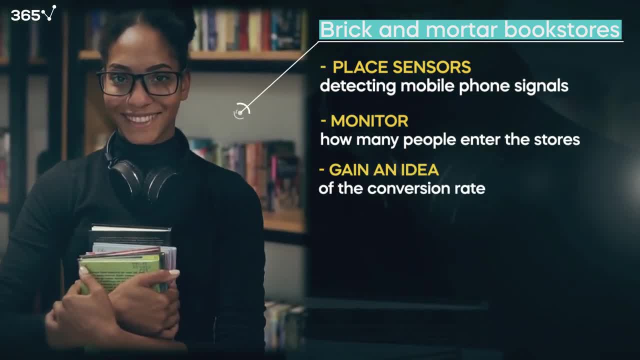 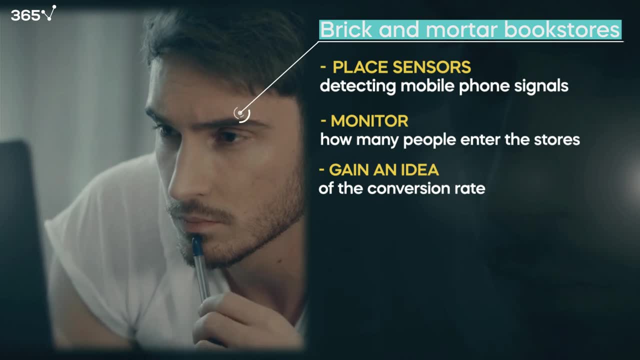 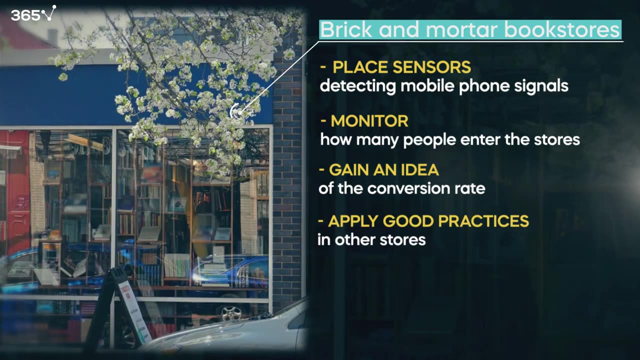 Combine the collected information with the number of store visitors who end up purchasing one or more books. In this way, management will be able to gain an idea of the conversion rate for each store and explore whether this benchmark is consistent across all three locations. Use the insights to understand if and why one location is doing much better than the rest. 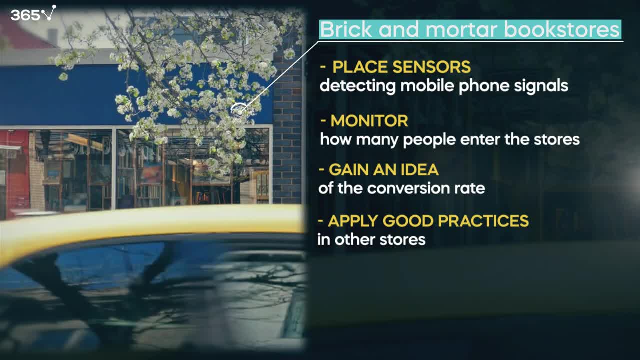 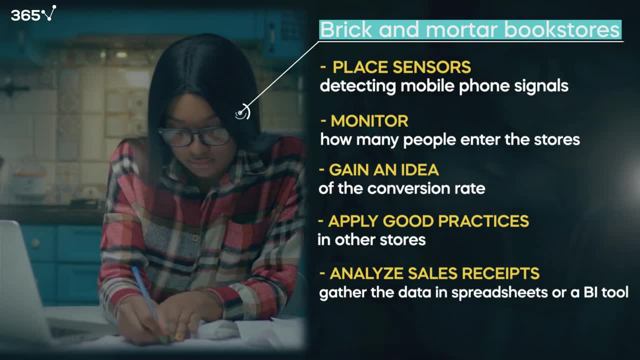 and then apply these good practices in the other stores as well. Analyze sales, collect sales receipts and gather the data in spreadsheets or a BI tool in order to find the relationship between store discounts and volume sold, thus gaining an idea about. 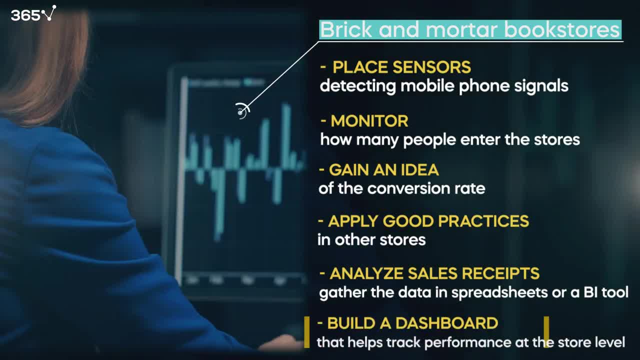 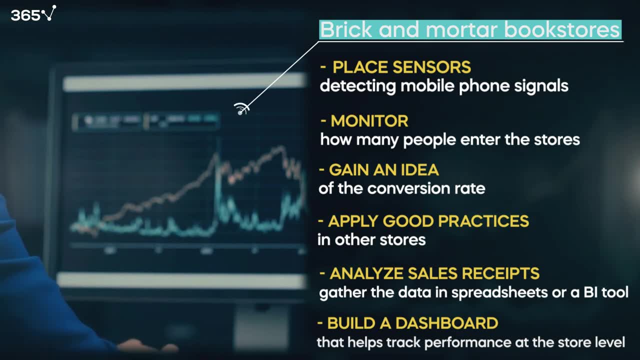 price sensitivity And, lastly, build a dashboard that helps track performance at the store level and shows how different genres and types of promotions are performing throughout the year. Data dashboards help employees work towards specific targets and hopefully this will help the team gain. 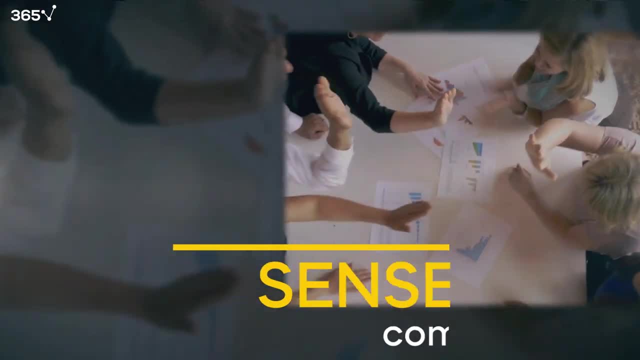 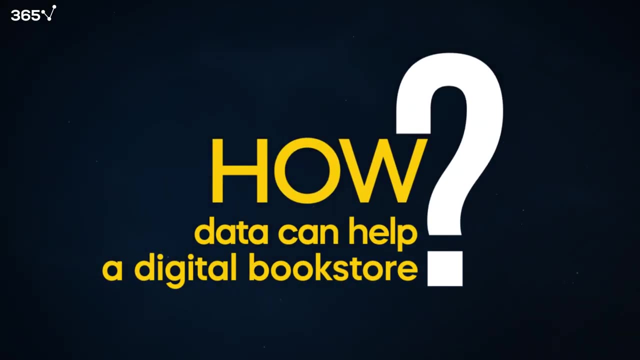 a sense of common purpose. Do you see how even-branded your product is? Do you see how even brick-and-mortar businesses can benefit from data-driven decision-making? Now let's consider how data can help the digital bookstore. Employing Google Analytics allows them to monitor incoming traffic and establish a conversion rate. 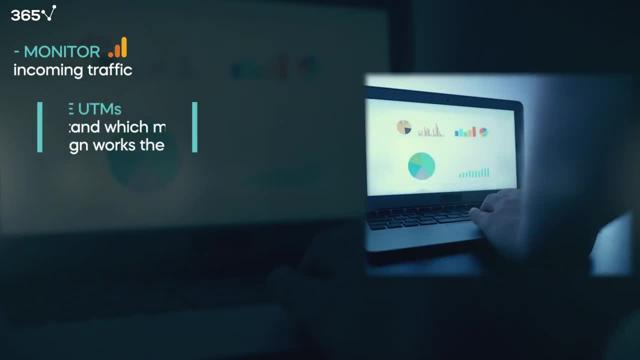 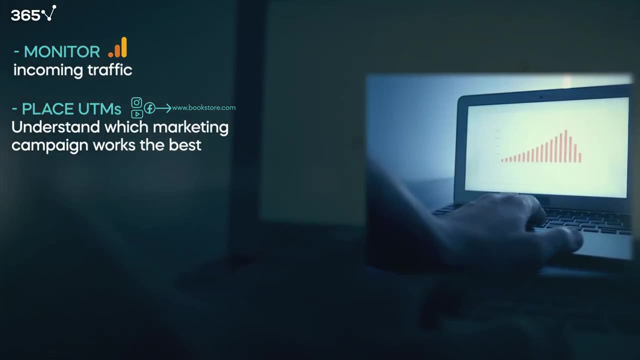 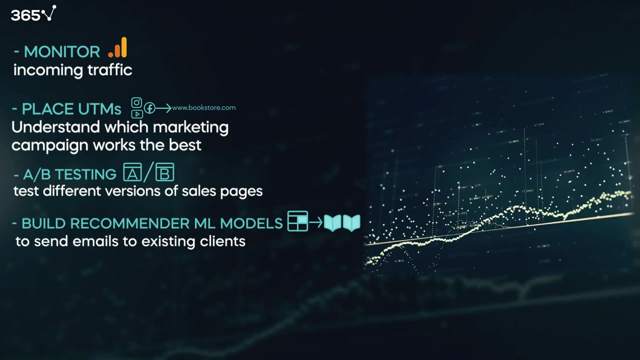 per unique website visitor. Placing UTMs to all external links to the website can help them understand which marketing, ad campaigns and social media efforts represent the best opportunity. Experimenting with different versions of sales pages through A-B testing, building recommender ML models that help them send emails to their existing clients with 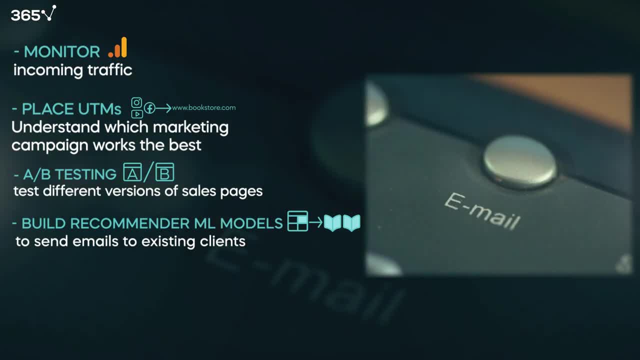 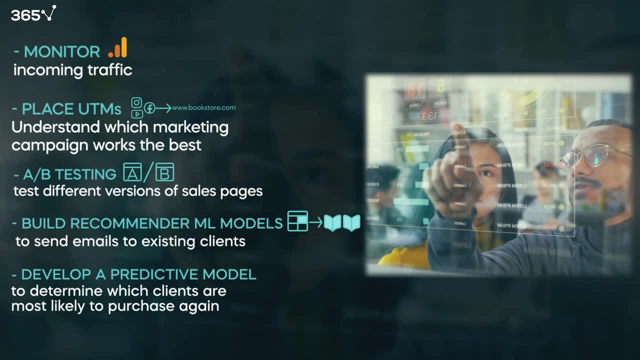 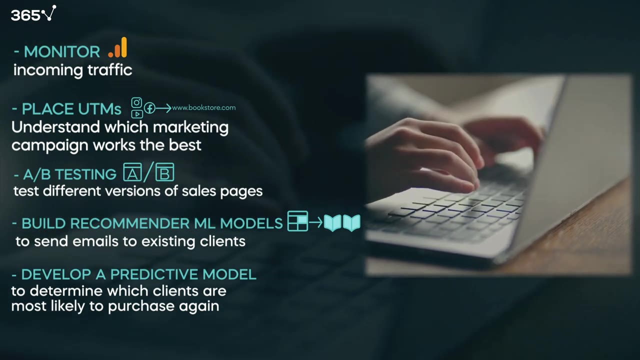 relevant book recommendations. increasing the chance of repeated purchases. Developing a predictive model based on demographic data and recorded interactions from the website to determine which clients are most likely to purchase again. The company can then use their emails for retargeting with Facebook, LinkedIn or Google.